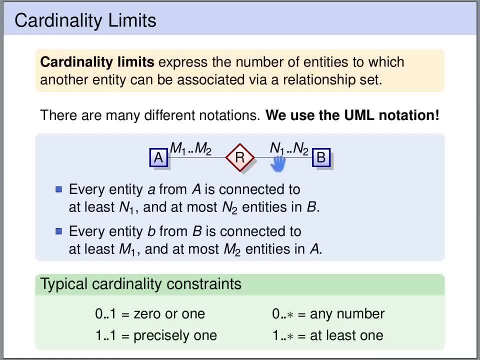 is related to at least a cardinality limit. So we annotate n1 and at most n2 entities from the set B. Likewise, the cardinality limit on the side of A- m1.m2, expresses that every entity from the entity set B. 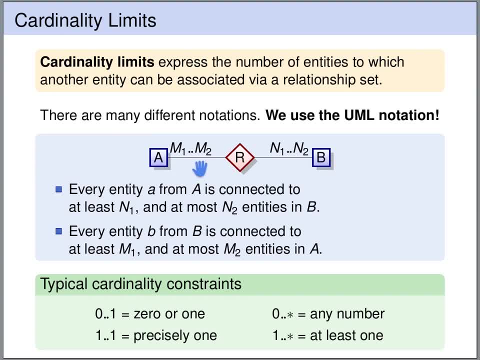 is related to at least m1 and at most m2 entities. from the entity set A. A number of typical constraints are: a number of typical constraints are: 0.1, expressing that it's related to 0 or 1. 0.0 star. we write for an arbitrary number. 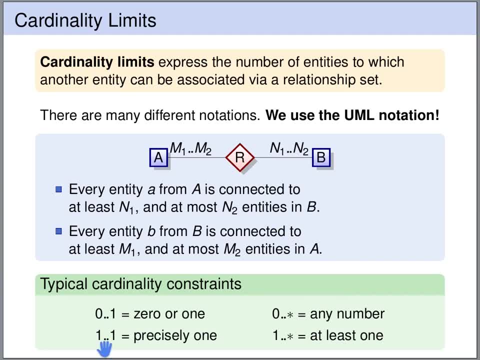 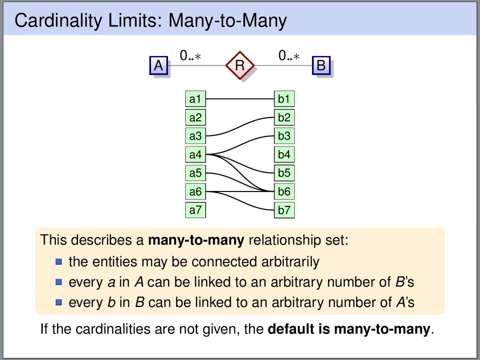 We write 1.1 for precisely 1, at least 1, and at most 1 gives you precisely 1.. And 1.0 star for at least 1.. Let's have a look at some examples. We can express a many-to-many relation. 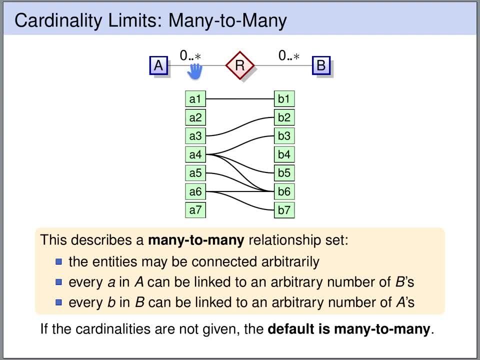 We can express a many-to-many relation by annotating both connections with 0.0 star. This expresses that every A is connected to an arbitrary number of B's and every B is connected to an arbitrary number of A's, So this is just an arbitrary relation between A and B. 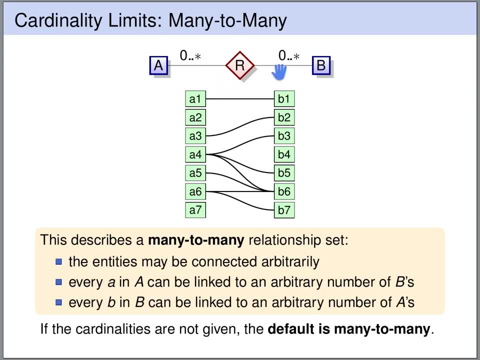 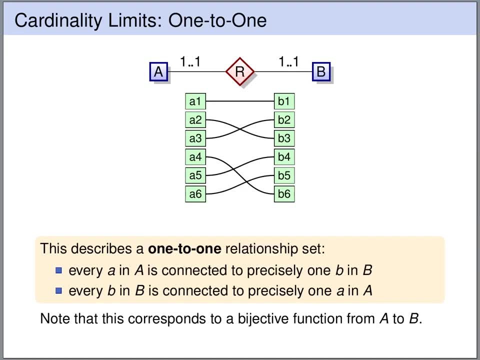 If the cardinality limits are not given, then this is the default. So the default is a many-to-many relation. If we annotate both connections by 1.0.1,, we get a one-to-one relation. This means that every A is related to precisely one B and every B is related to precisely one A. 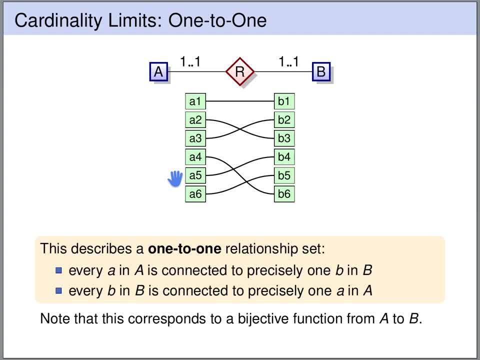 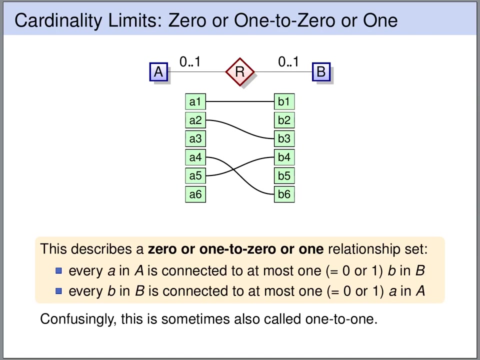 So in a mathematical sense, this gives you a bijection between A and B, And this also means that the entity sets A and B are related to precisely one. A And the entity sets A and B contain the same number of entities. We can express a 0-to-1-to-0-o-1 relation by annotating both connections with 0.0.1.. 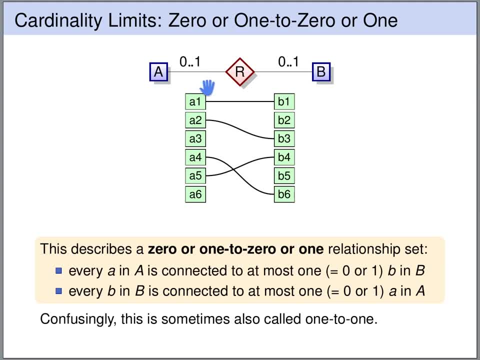 So by these cardinality limits we express that every A is related to 0 or 1 B's. So every A is related to at most one B. It can be related to one like a1.. A2 will be related to a3.. 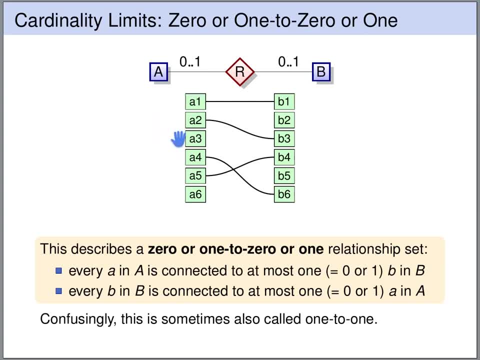 A4 will be related to a5.. also related to 1, a3 is related to 0, a4 is related to 1, a5 is related to 1, a6 is related to 0. And likewise, every b is related to, at most, 1a. 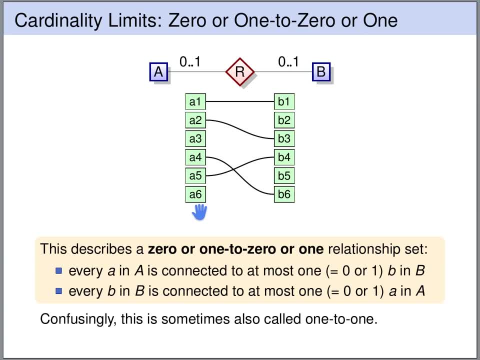 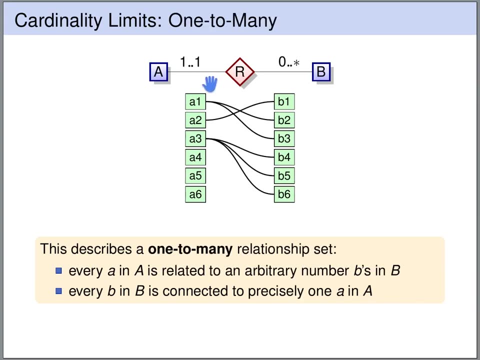 So this is a 0 to 1 to 0 or 1 relation. Confusingly, in the literature and on the web this is often also referred to as a 1 to 1 relation. We can express a 1 to many relation by annotating the one side by 1.1 and the many side by 0.0. 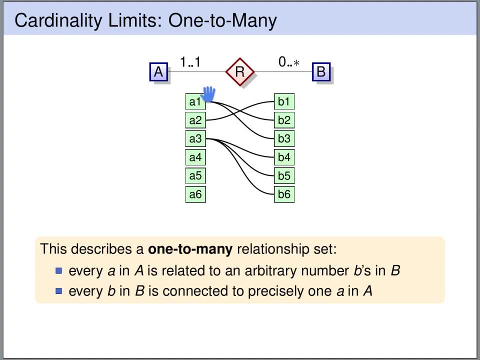 So we express that every a is related to an arbitrary amount of b's and every b is related to precisely 1a. So let's have a look: b1 is related to a2.. So, precisely 1a. b2 is related to a1.. 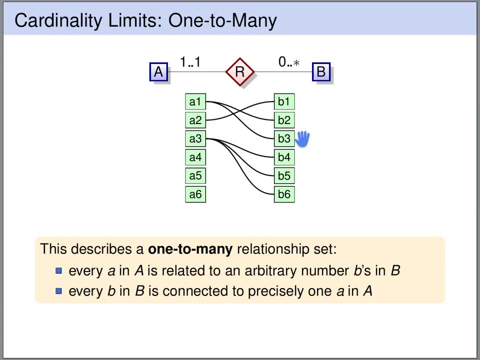 Precisely 1a. b3 is related to a1.. Also precisely 1a, And so on. If we want to express a 0 or 1 to many relation, we annotate the 0 or 1 side with 0.1 and the. 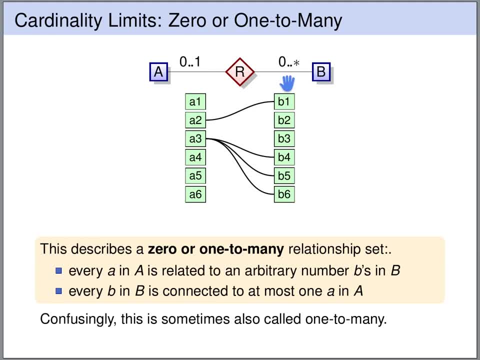 many side again with 0.0.. Now every a is still related, Every b is related to an arbitrary number of b's And every b is related to 0 or 1a's. So every b is related to at most 1a. 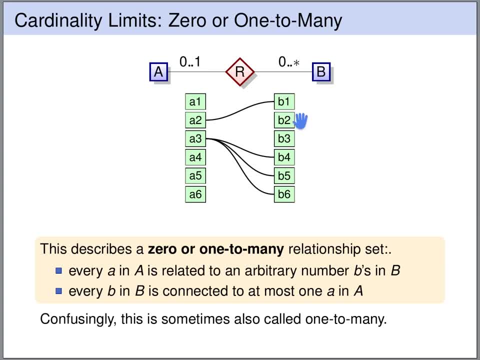 Let's have a look: b1 is related to 1a, b2 to 0,, b3 to 0,, b4 to 1,, b5 to 1, and so on. So this is a 0 or 1 to many relation. 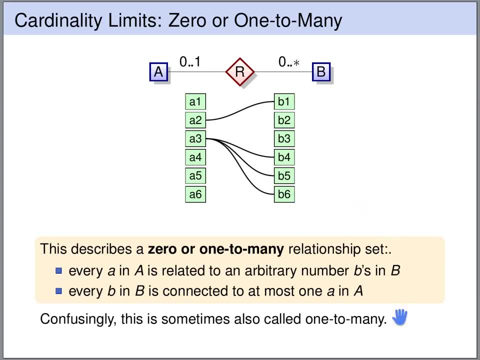 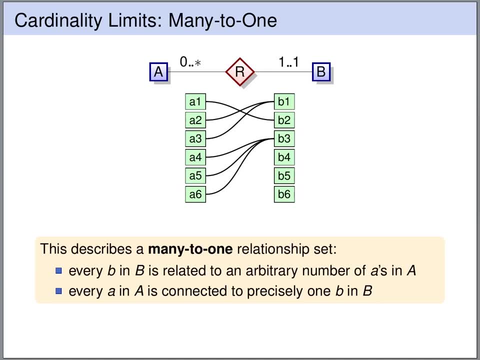 Confusingly. in the literature and on the web this is often called also a 1 to many relation. We've seen how to express 1 to many relations And of course we can also express the reverse, a many to 1 relation. 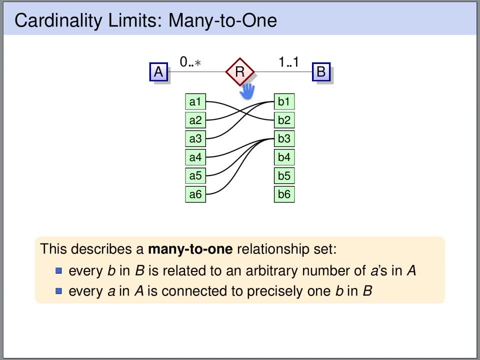 We simply annotate the many side by 0.0 star and the 1 side by 1.1, as before, It's just mirrored. now And now we express that every a is related to precisely 1b And every b is related to an arbitrary number of a's. 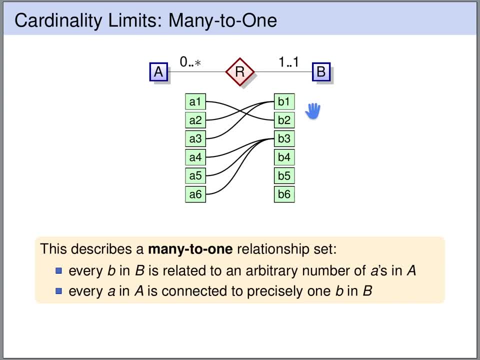 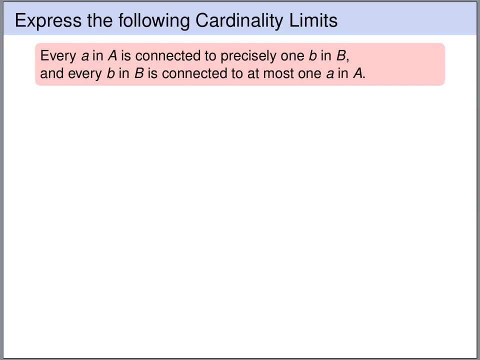 So this is just the same as before, The 1 to many just flipped around, And the same holds for many to 0 or 1.. It's just the mirrored version of 0 or 1 to many. Let's practice a bit with Coordinate Limits. 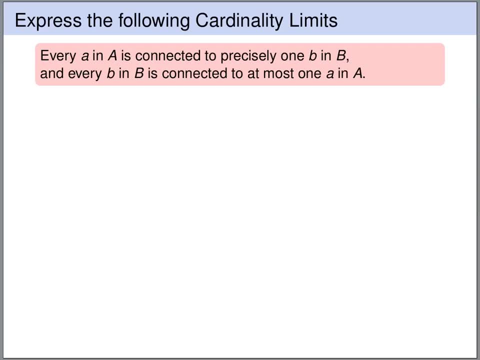 First, we want to express that every a is connected to precisely 1b. That means we have 1b. That means we have 1b, We have a Kal Observator. So how do we do that? First, we have to annotate the b side with 1.1, and we want to express that every b is: 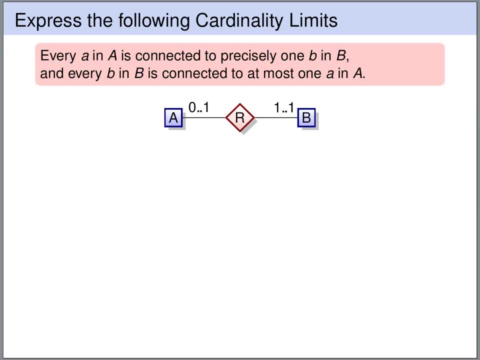 connected to at most 1a. So we annotate the a side with 0.1.. Next, we want to express that every a is connected to one or more bs, So we annotate the b side with 1.4 star, and every b should be connected to at most 1a och 0 .1ha, and every b should be connected to at most 1a. so every fear'll all the into Rah let As x's and Had As Ner Freqs an Odell km listeners routine呵 scripture Koos ret. Whoever you see in this back- hearings and going forward, it is up to you. 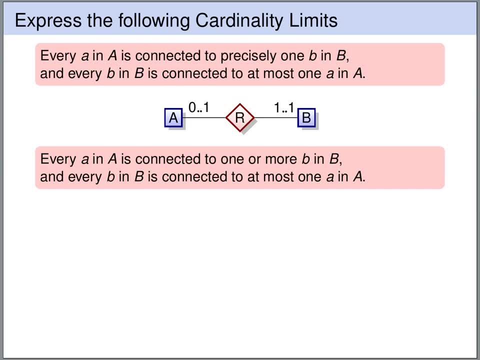 The Oz belonging to the root solution, rather than Kim altro B, proveing to that critical Bh. this is absolute R패Nab healthy, So we annotate the A-side with 0.1.. Finally, we want to express that every A is connected to one or more B. 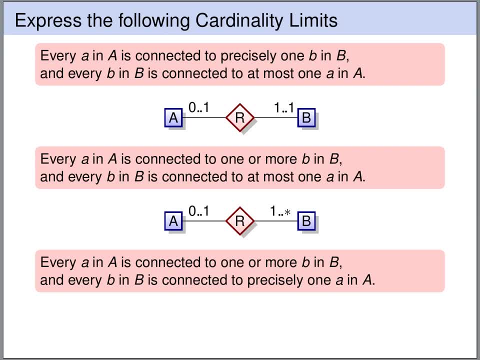 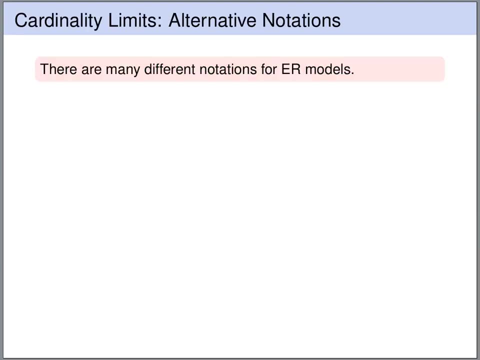 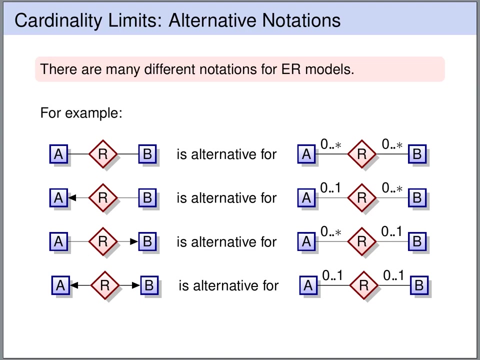 We again annotate the B-side with 1.0.. And every B is connected to precisely one A, So we annotate the A-side with 1.1.. There's many different notations for the cardinalities in Entity Relationship Diagrams. One alternative, for example, is that we use these arrows to express 0 or 1.. 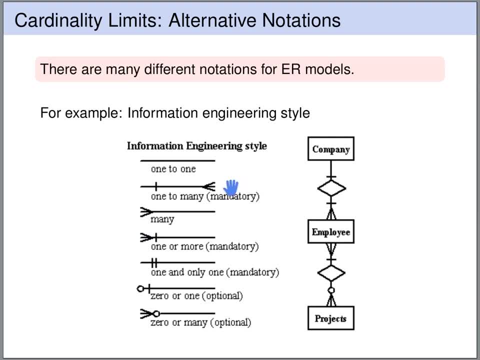 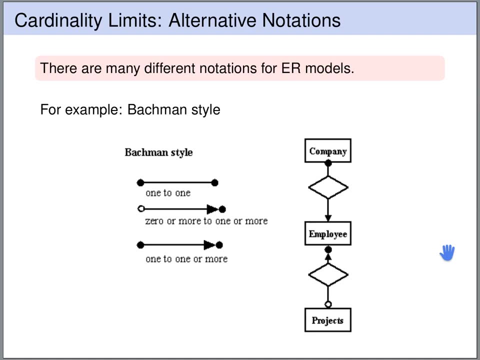 The engineering style uses such fans to express many and it uses such a circle to express possibly 0. There's a Chen style, there's a Bachmann style, there's a Martin style, and this style is closest to what we are using.